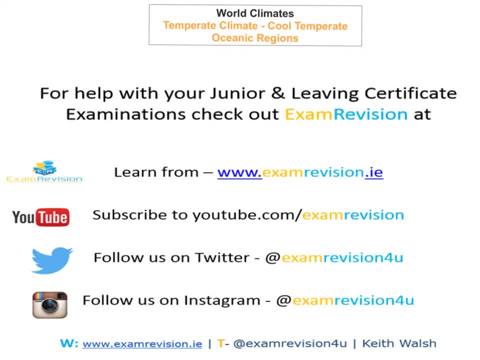 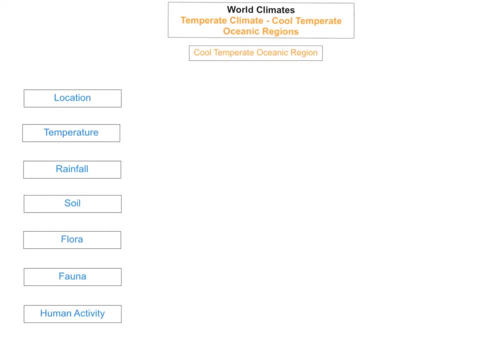 And we're going to look at the cool temperate oceanic climate. So we're going to focus on the cool temperate oceanic climate of a region And the first thing you'll need to know is where you can find, whereabouts is the cool temperate oceanic regions located? 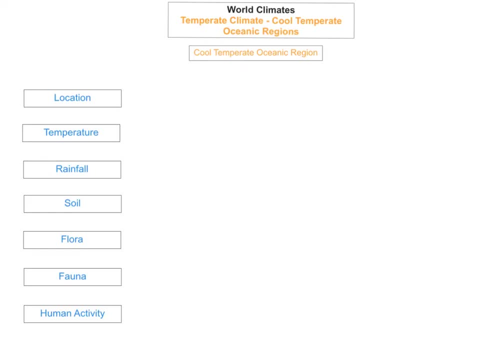 And they're located mainly between 40 and 60 degrees north and south of the equator, So mainly 40. And then 40. And then 40. And then 40. And 60 degrees north and south of the equator. 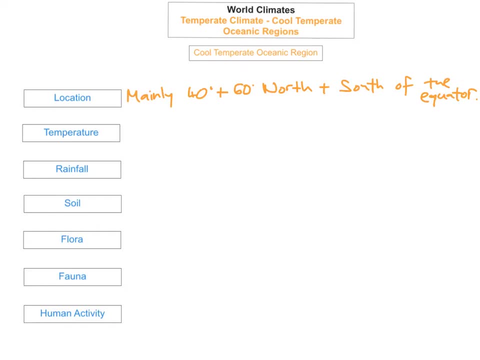 So an example would be Ireland in the Northern Hemisphere and the Southern Hemisphere. So an example would be Ireland in the Northern Hemisphere and the Southern Hemisphere. You could pick New Zealand. The temperature: Winters are generally cold. So winters are generally cold. 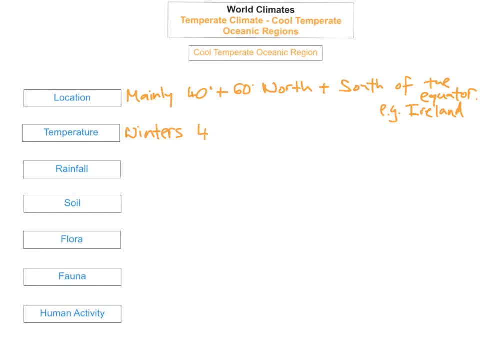 And temperatures are about 4 degrees Celsius to about 7 degrees Celsius, And the summer Are generally cool, With temperatures going from about 14 degrees Celsius to 16 degrees Celsius. The next one we're going to look at is the rainfall. 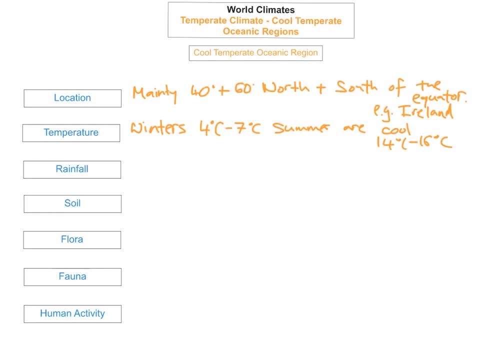 And rain is experienced throughout the year, And in Ireland, In the west of Ireland. So in the west of Ireland They receive Around 2.5 degrees Celsius thousand millimeters of rain, of precipitation, each year. in the east, however, we only, they only- 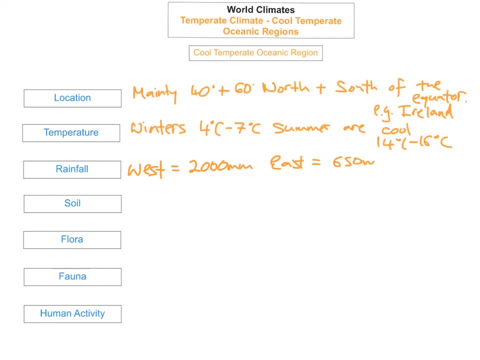 receive 650 millimeters uh per year and this is due to uh the rain being carried by the winds um from the sea, and that is why a lot of we get a lot of relief rainfall on the west, and that's where they receive um nearly three times the amount of the east of ireland soil type um. 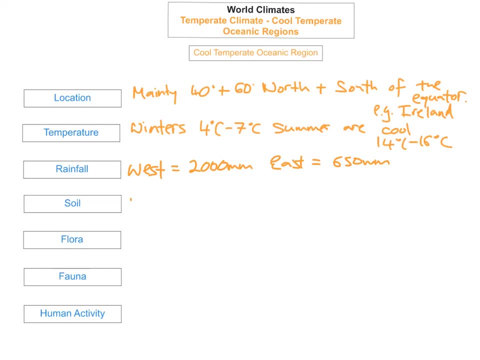 the soil is very, uh, very fertile. you've got very fertile soils and the main soil they can find in this region is the brown earth soils. so it's really good for agriculture, really good for farming and growing crops. so the brown earth soils, um um the floor, it's a mixed um. 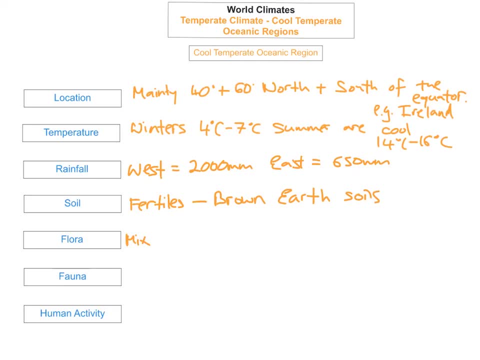 of like deciduous and cniferous like forests, so mixed of deciduous and cniferous forests um you'll find many different species of plants. you'll find many different species of plants, including like ash, elm and oak, and lots of natural vegetation can be found. 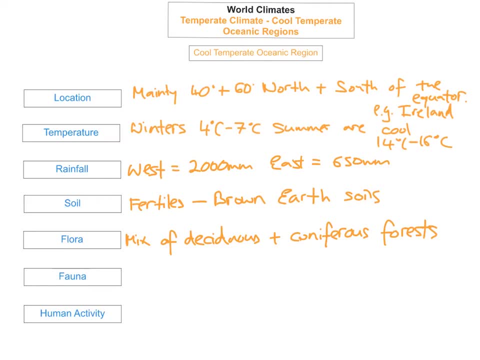 here, unless it's been cleared for agriculture or for, maybe, cities and buildings. The next one is the fauna, and you'll find many different animals in this region. A few typical animals that you might find here might be deer, fox, badgers, squirrels, etc. In this region you'll find lots of. 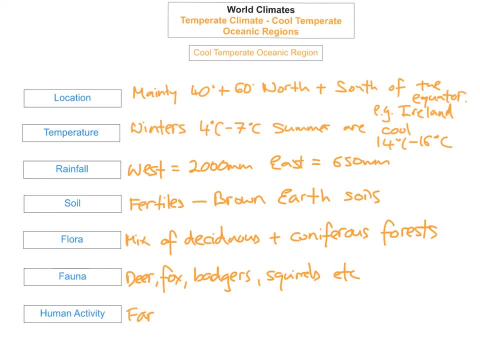 human activity, where humans will be farming the land, so there will be lots of agriculture. You'll find lots of animals in the fauna and you'll find lots of animals in the fauna and you'll find lots of animals in the fauna and you'll find. 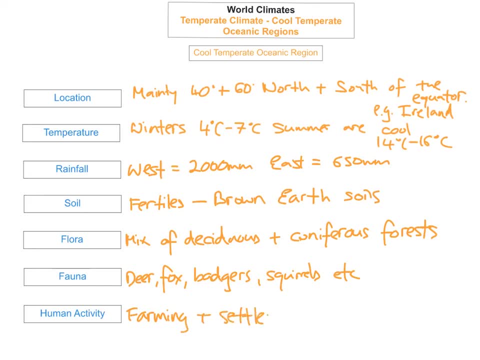 lots of settlements, and settlements tends to happen more over in the east side of Ireland, and this is due to the more favourable climate because they receive like less rainfall. In most of Ireland, you'll find like widespread of like of farming. however, though, because of the abundance of brown, 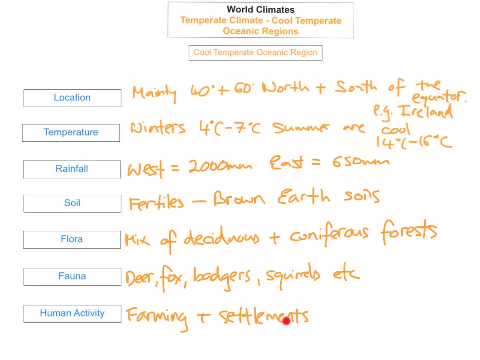 earth soils, which makes growing of crops and the farming of land and very popular and profitable. growing of crops and the farming of land and very popular and profitable. Okay, so that's it for today's tutorial. we've looked at cool temperate Oceanic region. An example of a cool temperate Oceanic region they can find is Ireland.